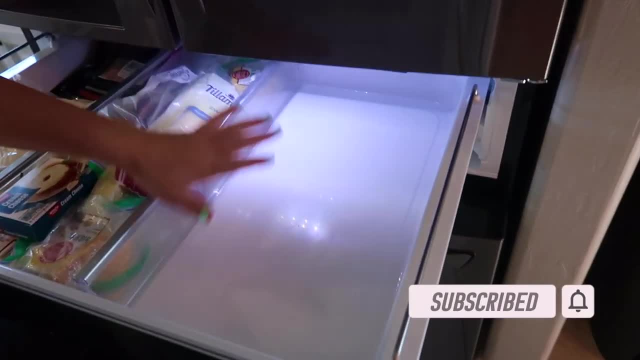 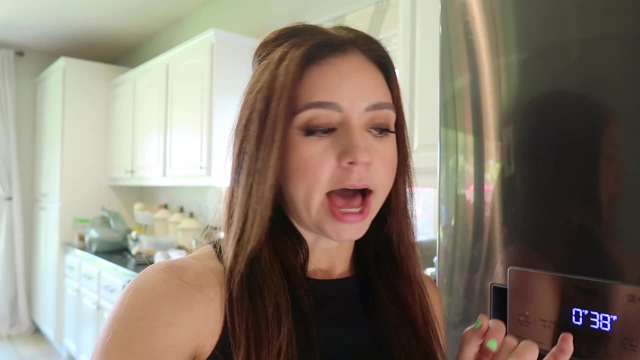 You can pull this out and this side is where everything is going to be at. So anything that they would like is going to be on this side of the fridge, And what I'm going to do is I'm going to try to make it as organized as possible by using some Tupperware. So I already have these. 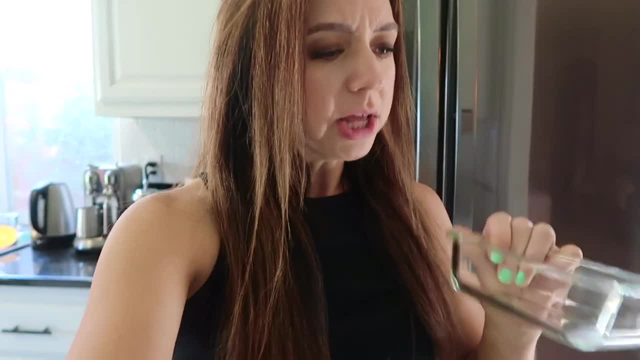 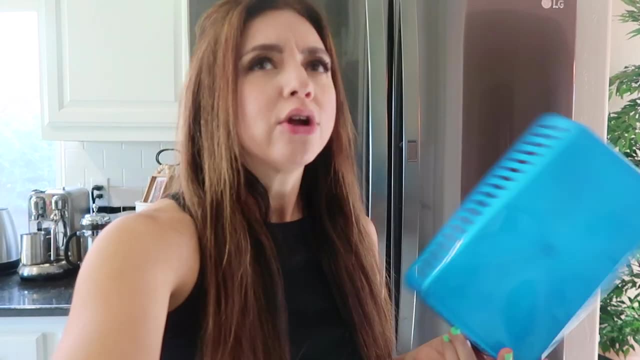 I don't really use these that much like the smaller ones, So I'm going to use these to try to make it all organized, And I also have this right here. I used this in a prior video. I think it was like a pantry organization video. I bought too many. 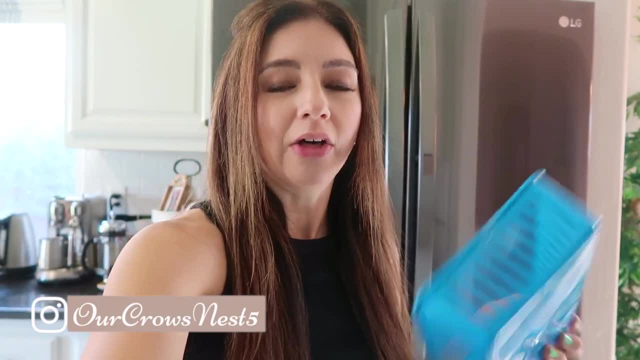 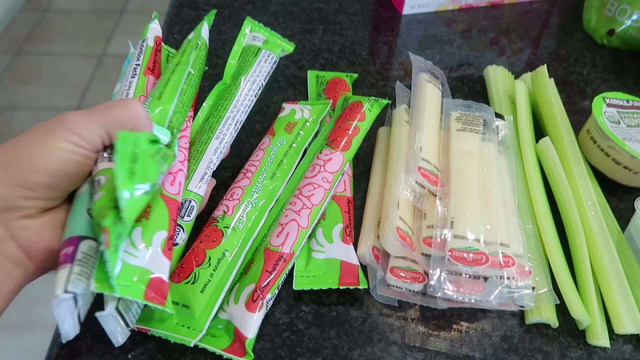 And I found this, So this is going to be perfect. if I need it, I'll slide that in there as well. So let me show you the snacks that I'm going to be putting in here. So I will be including some squeezy yogurts. I have some left over from my Trader Joe's haul, And then I'm supplementing. 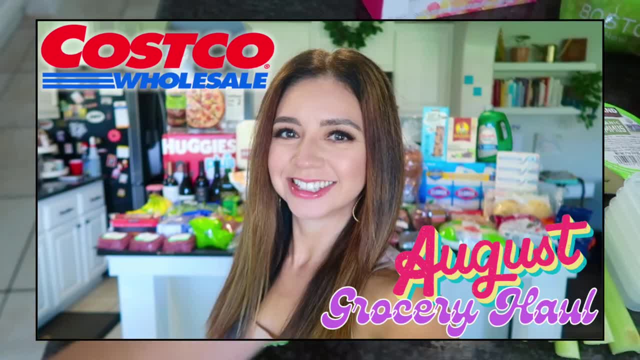 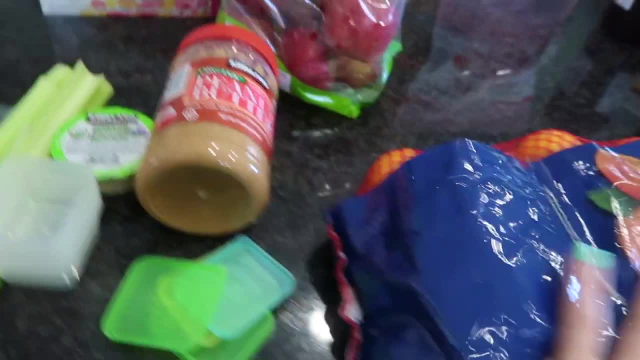 with some from my latest Costco haul That's going to go in there, along with some string cheese. I have some celery- I'll explain in a second- Some hummus, peanut butter, some oranges and then some apples. So what I'm going to do is I have these. 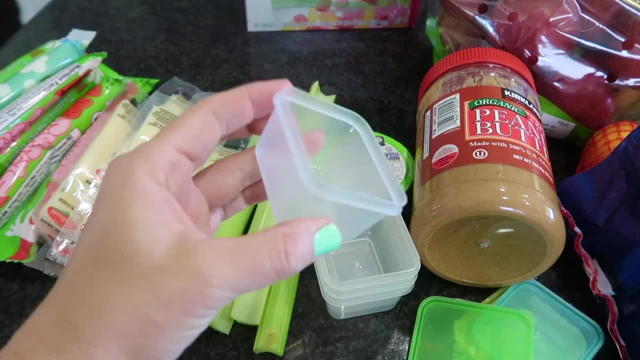 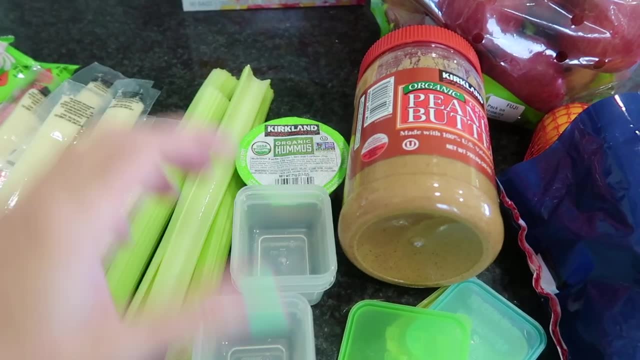 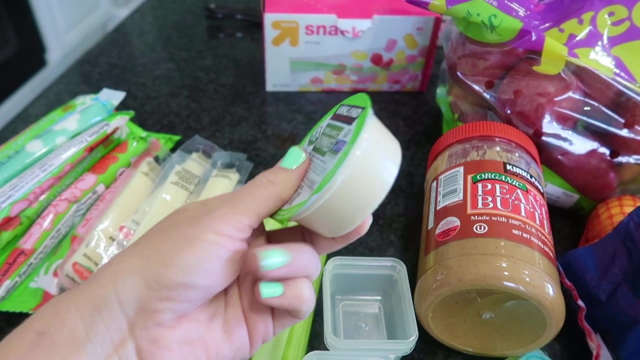 little tuppers. They're like really, really tiny, like dip sized, And what I'm going to do is I'm going to put some peanut butter in two of them And then in the other two, I'm going to actually divvy up this hummus. So I got these hummus cups from Costco. Now I find that these are a good 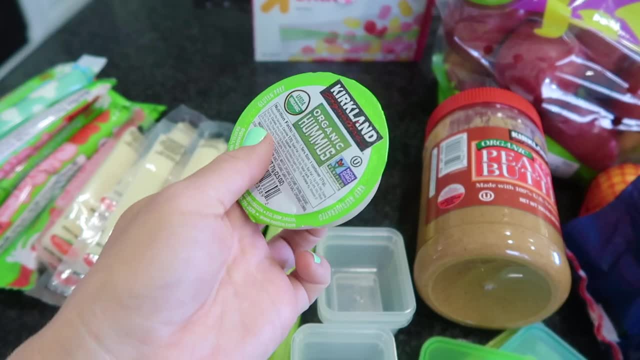 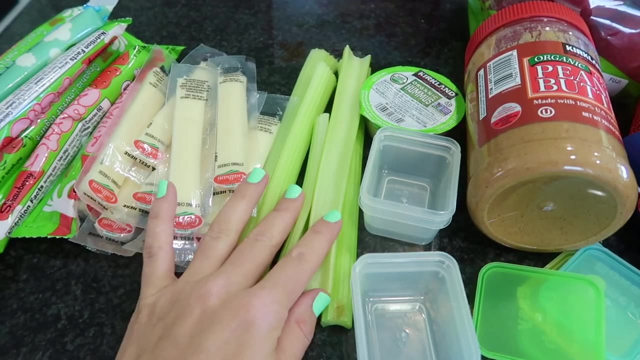 size for adults, but for kids? my kids always eat half of it, So I'm going to divide this up and put the hummus into two of these. So hummus is going to go with the celery sticks, And then I'm going 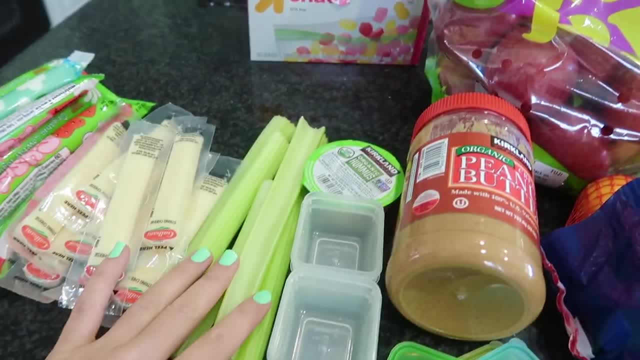 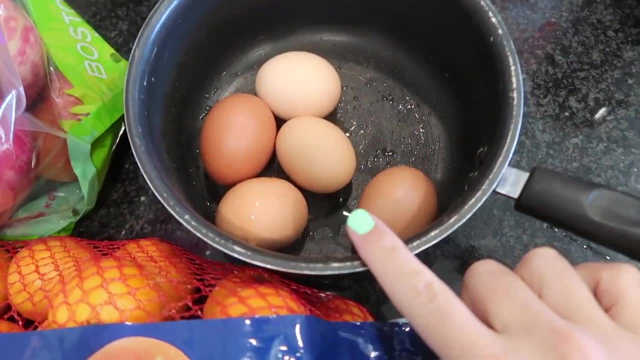 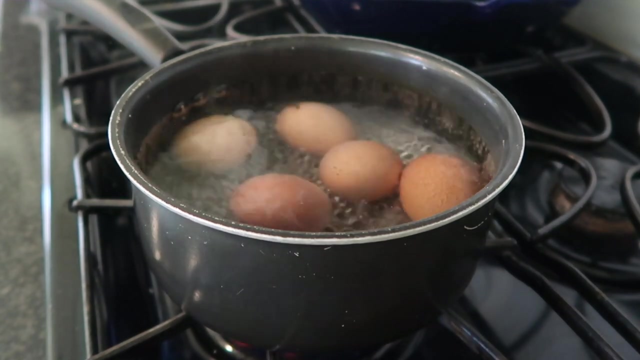 to put in here for some apples, or they can use a celery sticks as well. So this is kind of like for whatever they want to do. And then over here I do have some hard boiled eggs. All I did for the hard boiled eggs was I put these in cold water, I brought them up to a boil, I put a lid on top. 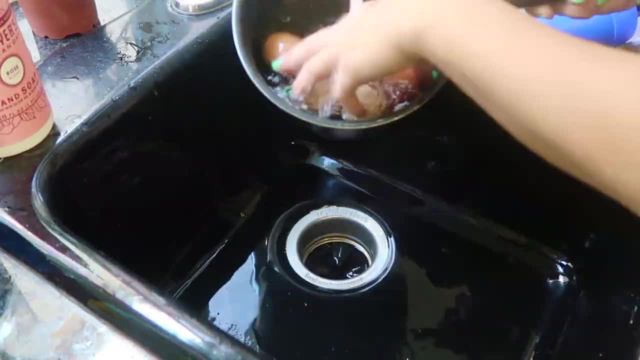 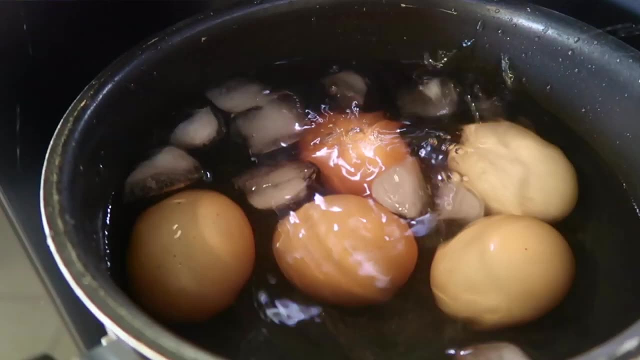 and I set a timer for nine minutes And then I rinsed these in cold water and I've added some ice to help cool them down And I let them sit there for about six-ish minutes or so And I'm going to keep them just like this, with the shell on, because it lasts longer if you keep. 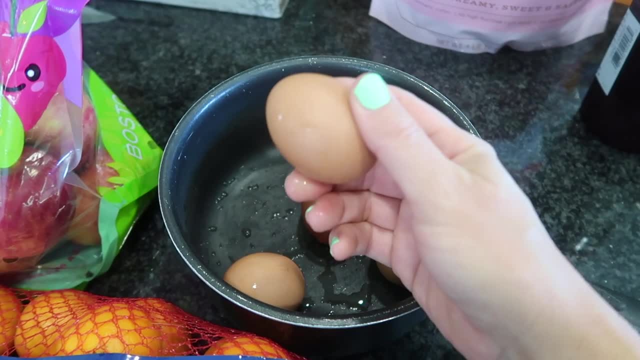 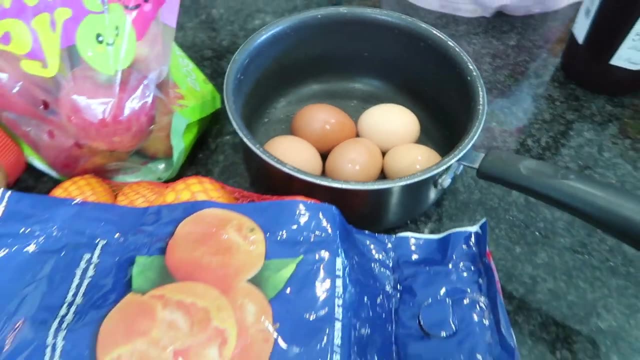 the shell on. I believe it's up to a week, but if you crack them and peel them, I think it's only like five. I think it's four to five days, but I'm going to leave them on just like that. So this is. 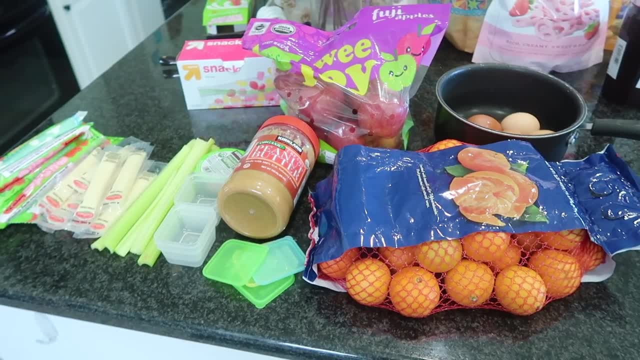 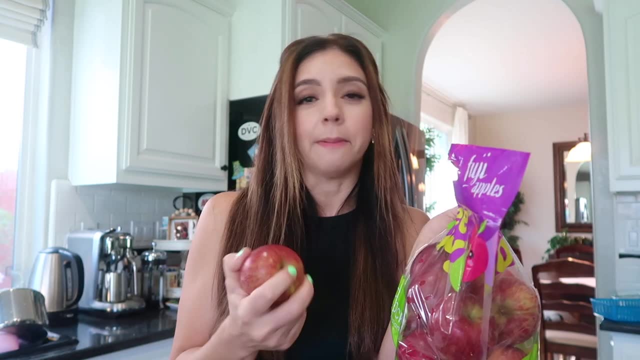 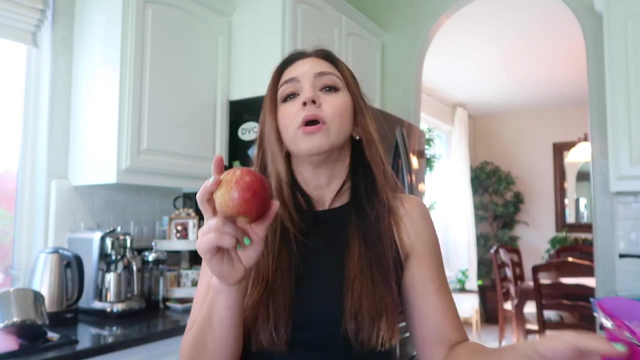 all of the snacks for the fridge and I'm going to start prepping it. I originally bought these apples from Costco- the small ones- with the intention of leaving them whole so they can just for them, so that they can dip it in peanut butter. So I want to do that right now And to make these. 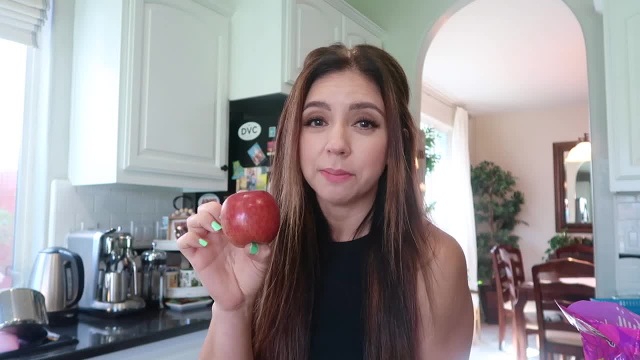 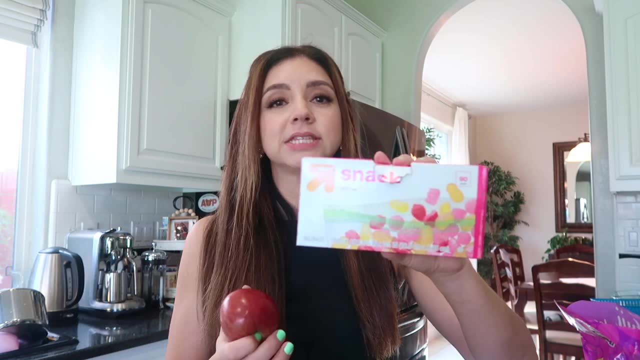 last longer. you want to slice them and submerge them in salt water for about five minutes or so to make them last longer. They won't brown either, And then I'm going to put them in little snack baggies. You can either use these plastic ones or, if you find, some small reusable ones, 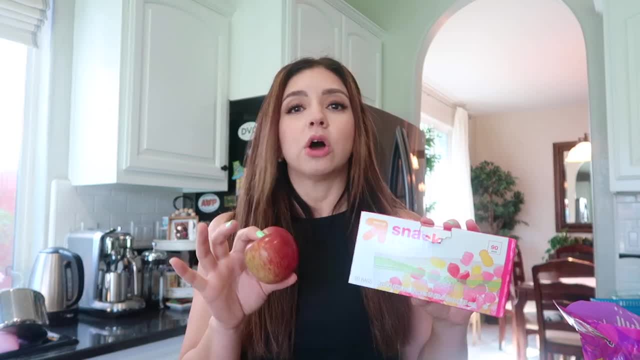 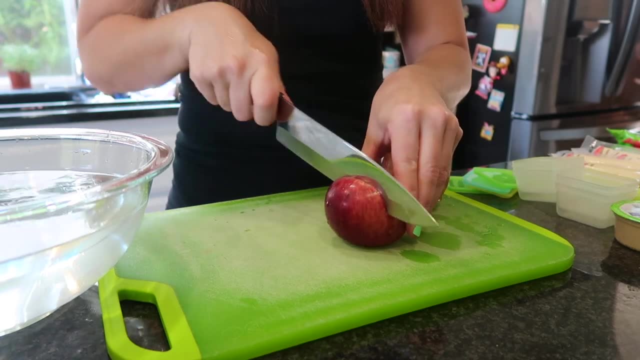 which these are reusable too. You can just rinse them out. They'll be good to go. So that's what I'm going to do right now. I'm going to prep my apples and start putting everything in the fridge. If you are new to my channel, I am so glad that you are here. My name is Alicia. 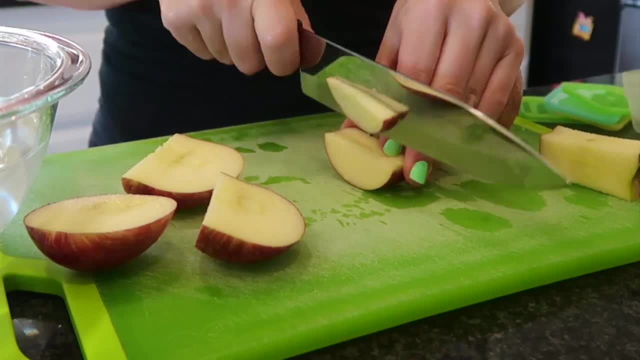 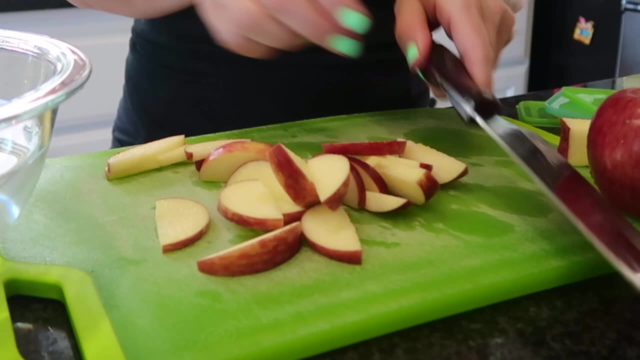 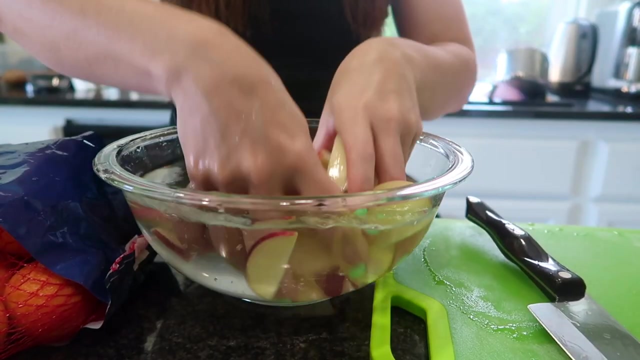 We are a family of five. I have two boys and one daughter. I've been with my husband for many, many years now. We've been married for 16 years already- It's crazy- And then together for 19,. I believe- Even crazier to me, But on my channel you can expect to find a lot of food videos. I 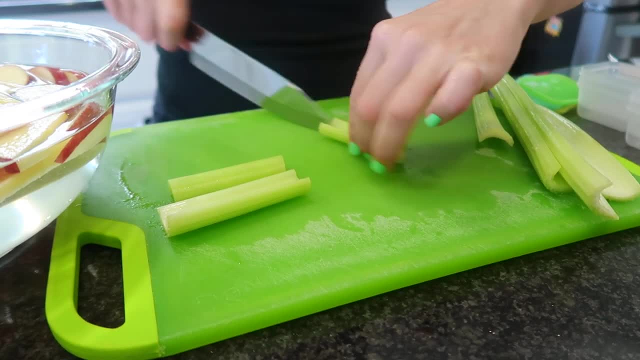 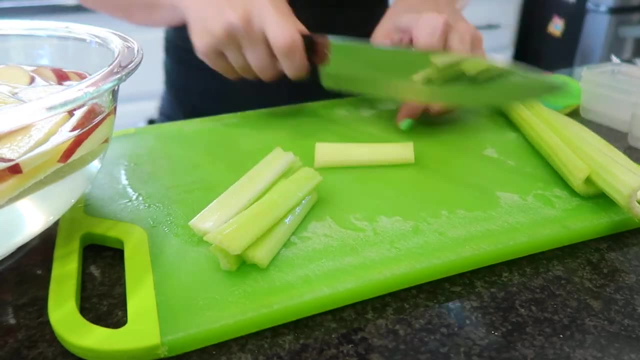 love doing grocery hauling. I love doing grocery hauling. I love doing grocery hauling. I love cooking, I love baking, I love doing all the food stuff. So you will find a lot of that here, And you will also find some Disney content. I love Disneyland and Disney World. We are DVC. 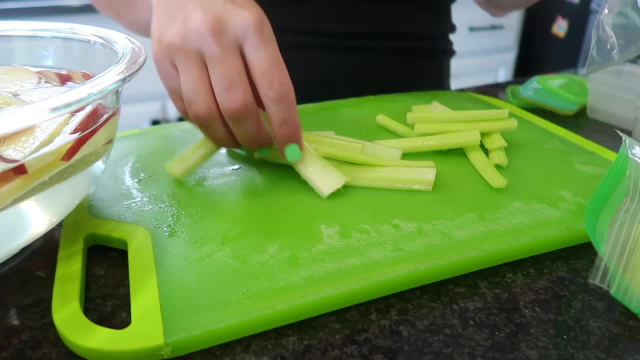 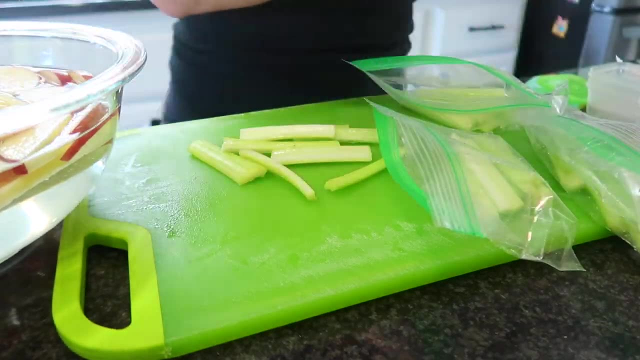 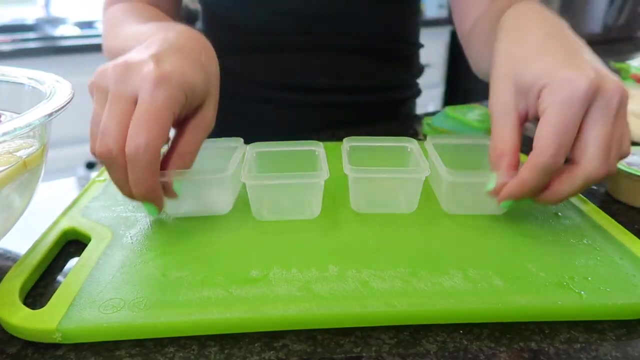 members, So we're kind of forced to go to Disney on our vacations. But you'll also find just some other fun family things And I have some more ideas coming up. So if you are new and you are not subscribed yet, please definitely subscribe to my channel so you can see other future videos. 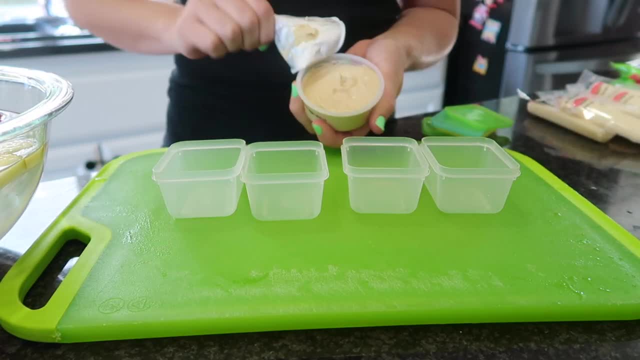 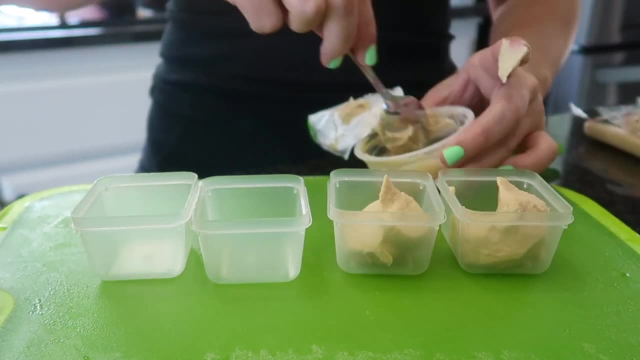 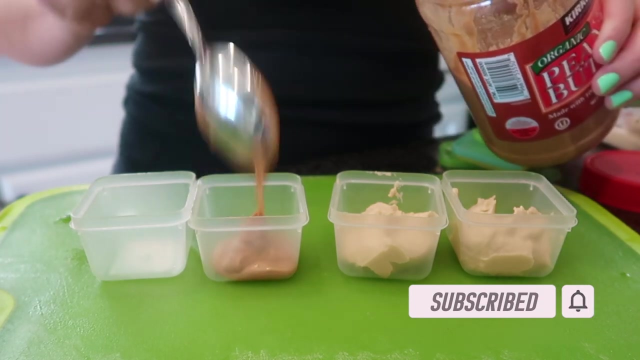 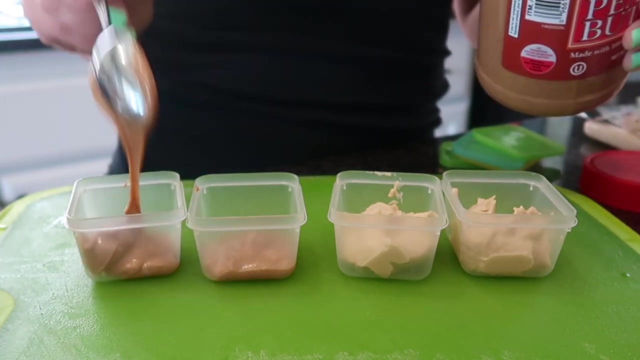 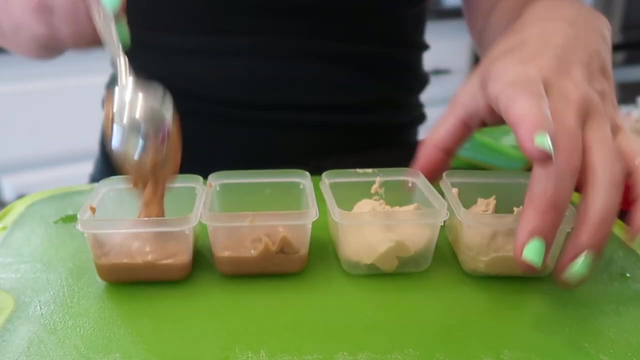 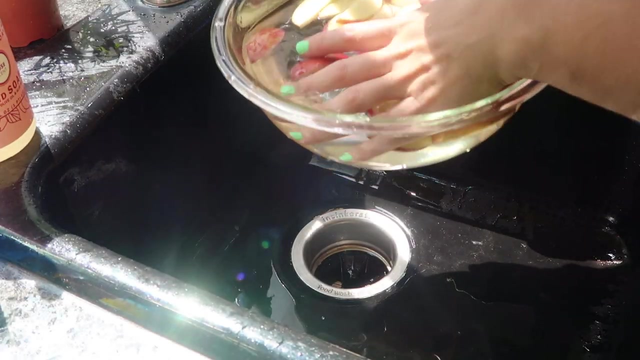 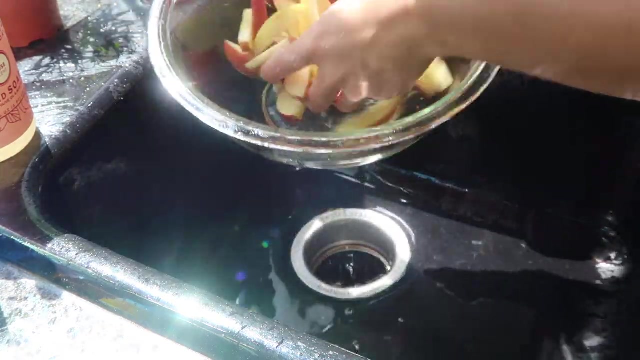 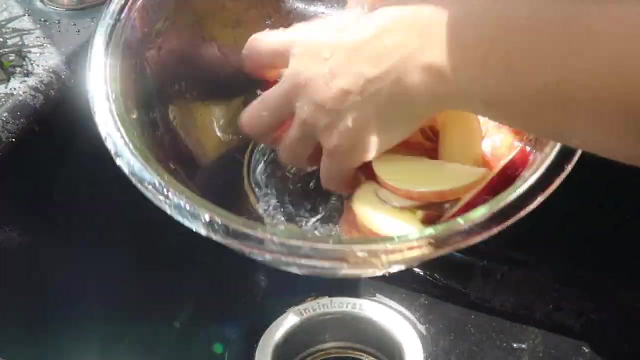 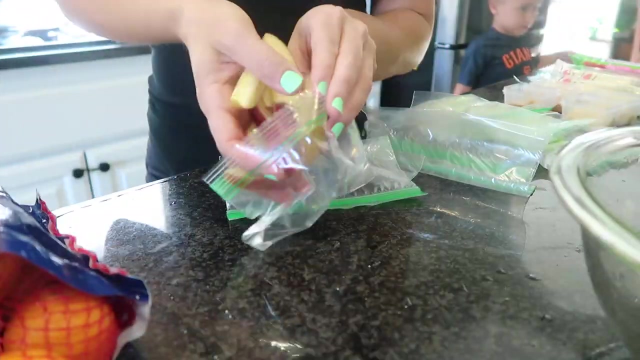 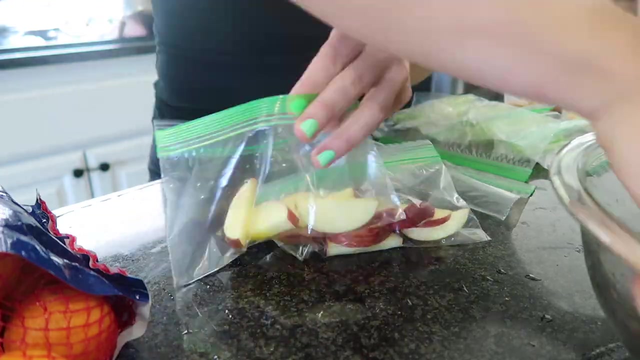 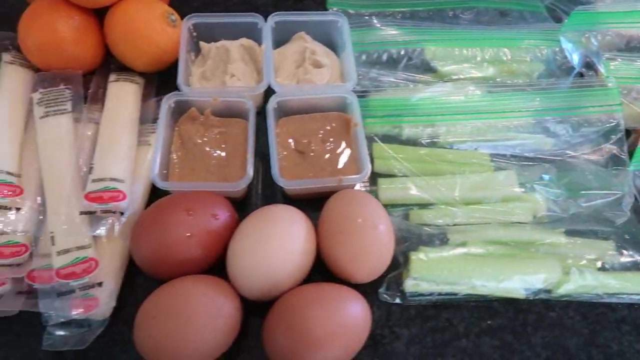 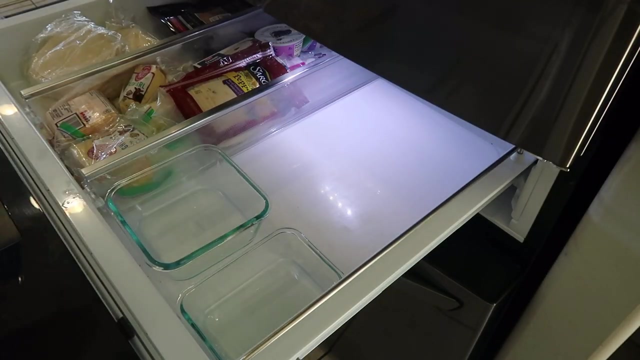 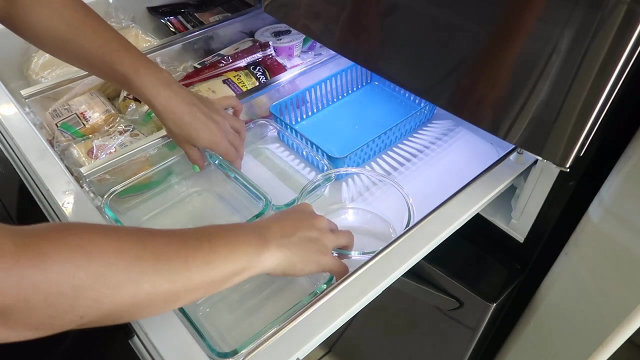 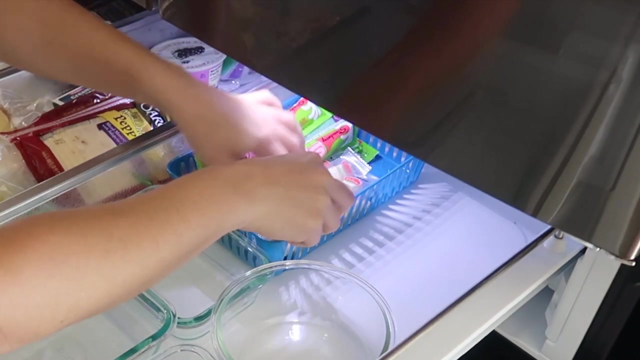 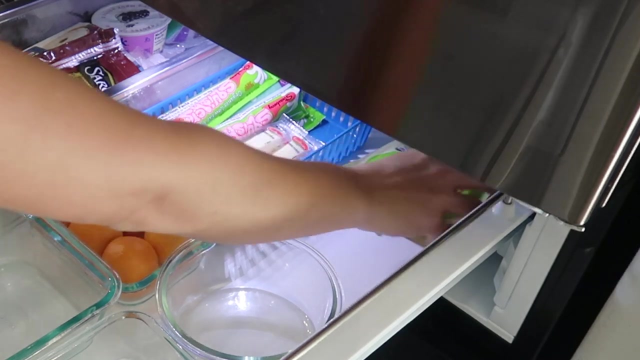 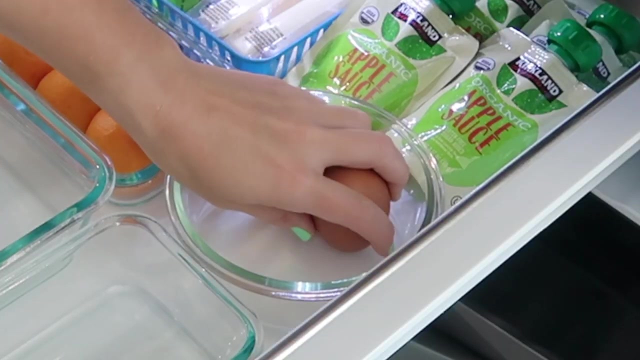 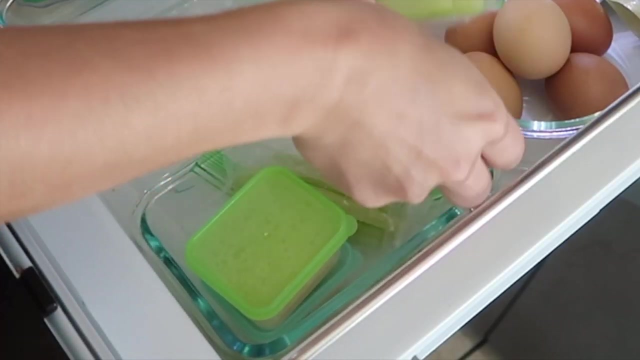 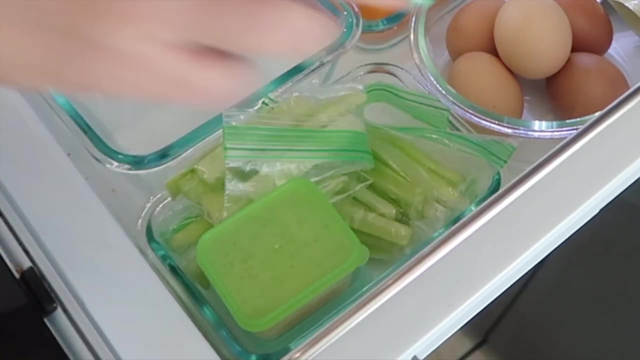 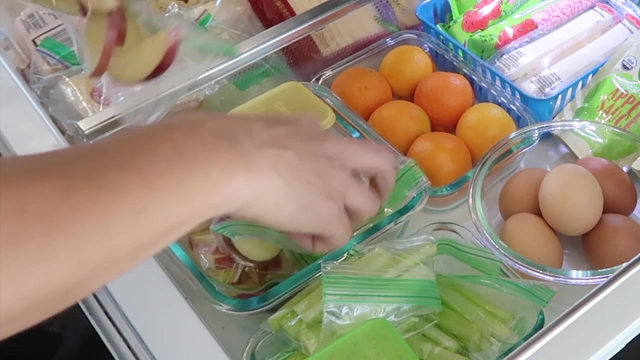 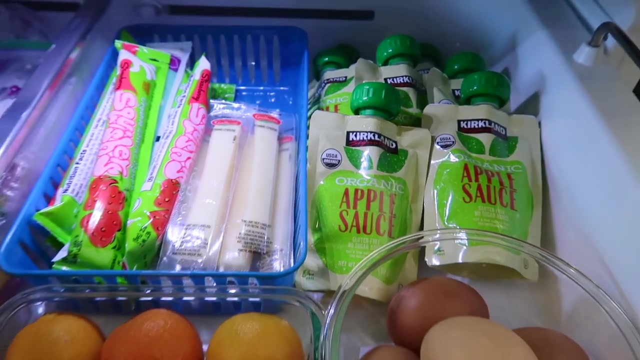 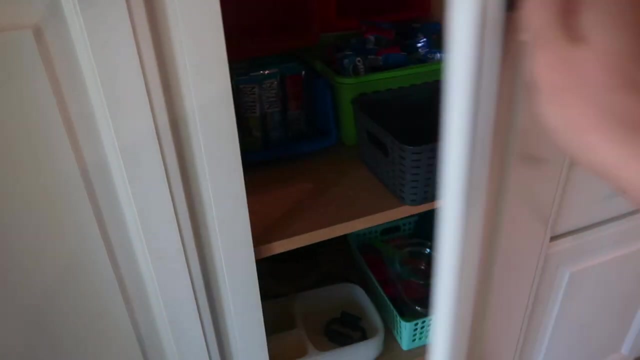 that are coming up. Thank you so much for watching. I'll see you in the next video. Bye. 🎵. Outro Music 🎵. 🎵. Outro Music 🎵. Alright, I wanted to show you the pantry area where I'm going to keep the snacks. It's pretty. 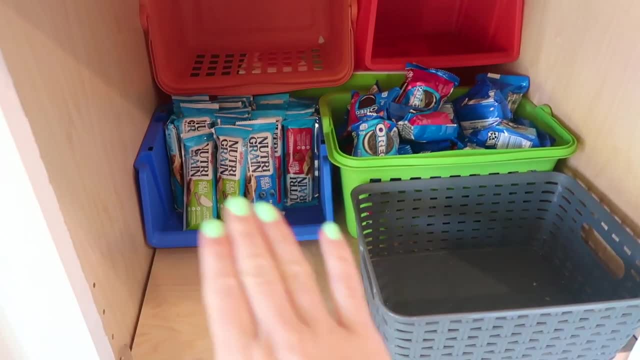 much cleaned out. I still have some Nutri-Grain bars over here. I'm going to keep them in the here that I'm going to keep there. And then these Oreos. I've had for a long time already, But they're. 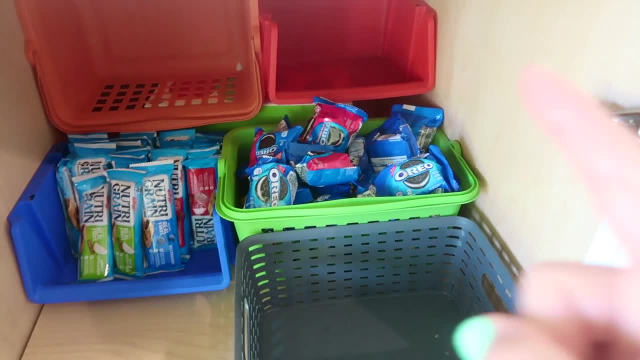 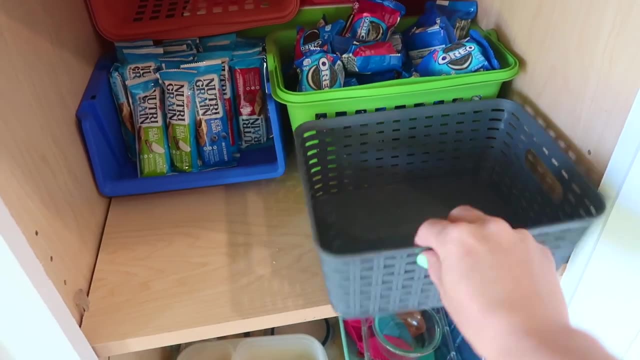 still good. I just checked the expiration date. They usually don't grab those. They know not to grab those because I will sometimes use those for their lunches, But I'm going to be filling up these empty guys right here. I got all of these, I think, from Dollar Tree, a long time ago And then back. 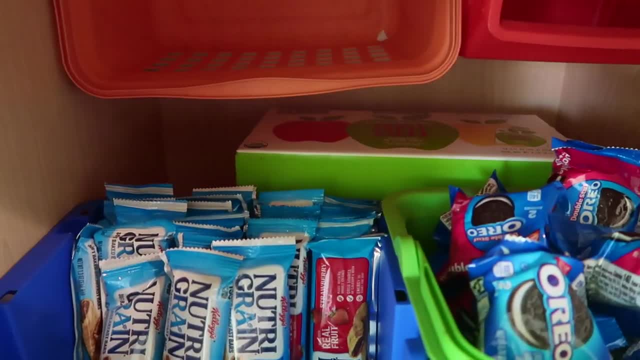 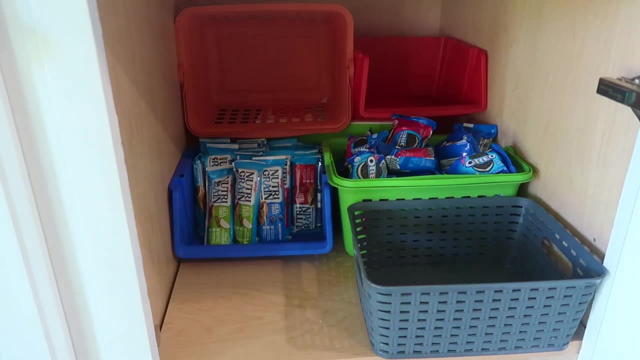 here because my pantry is so deep and you can't really see. I decided to use the applesauce box to put these guys on top so you can really see everything that's going on here. So I'm going to start prepping for the pantry And this is what I have for the pantry, What I'm 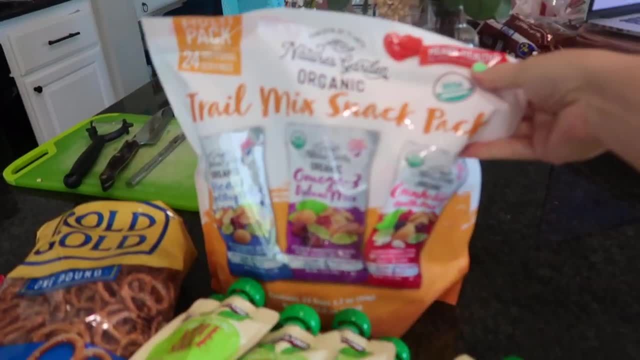 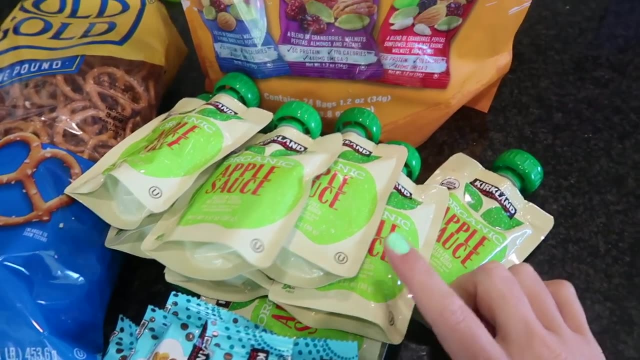 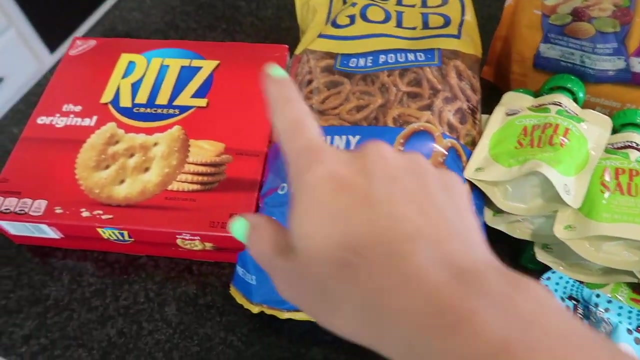 going to be adding so from Costco of course- is those little snack packs. I did put some applesauce in the fridge, but I am going to leave some out, I think as well, just for like room temperature ones. I have some of those soft and chewy chocolate chip granola bars, some pretzels and some Ritz. 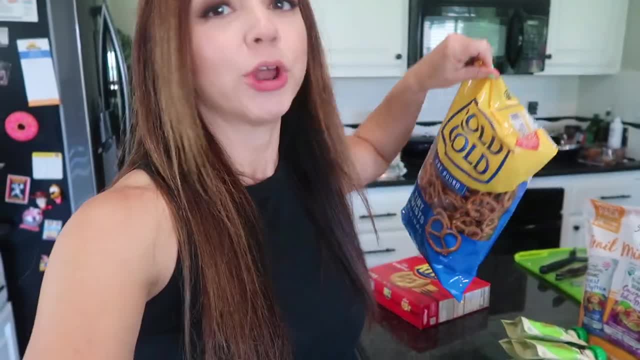 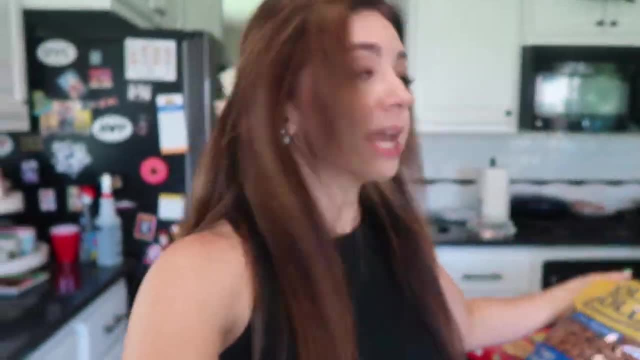 crackers. I'm obviously not going to just be putting like a whole bag of pretzels in the pantry, because that's going to be a lot of work, But I'm going to be putting a whole bag of pretzels in the pantry, So this is a very bad idea. These could be eaten in one sitting. Same with the. 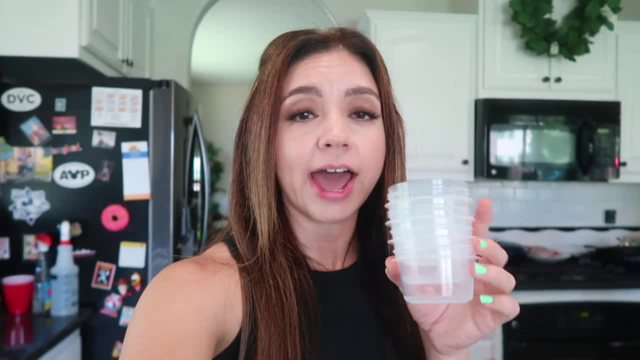 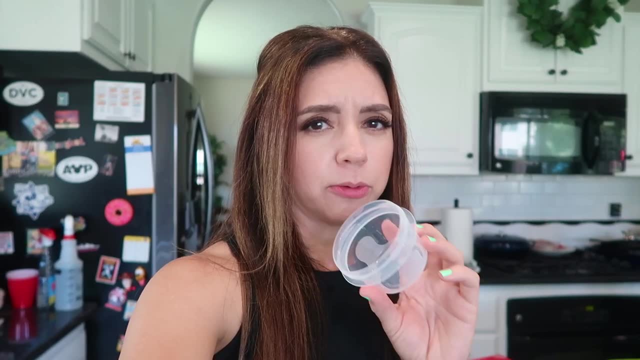 crackers, the Ritz crackers. So what I'm going to be doing is I have these little guys. They are like little reusable plastic sauce containers. I don't know where I got these from. I'll link some similar- but I use these all the time. What I'm going to do is I'm going to put pretzels in. 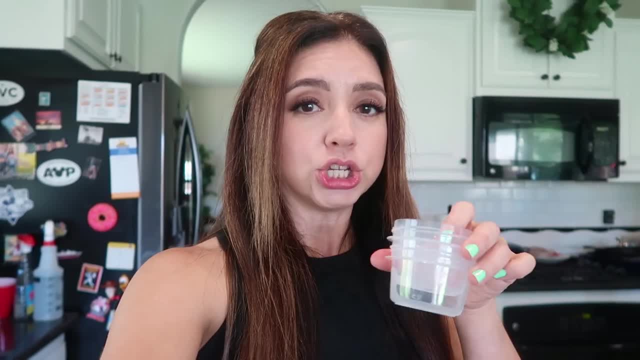 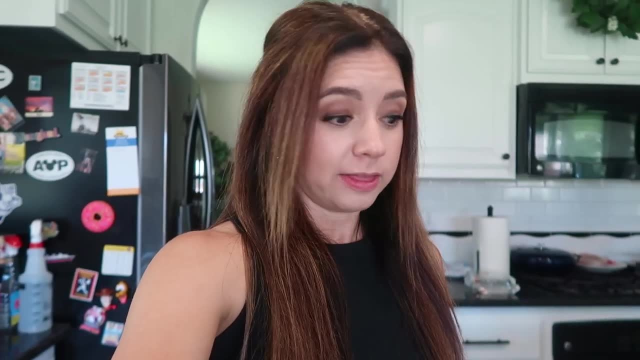 two of them. I have four right here, So I'll do pretzels in two, and then the other two I'm going to do Ritz crackers. So they don't get their hands in the bag, They don't eat everything that they. 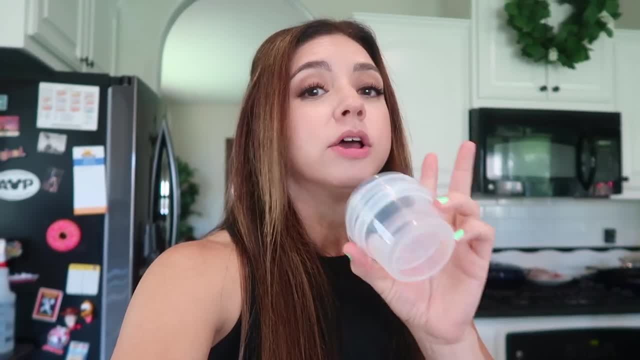 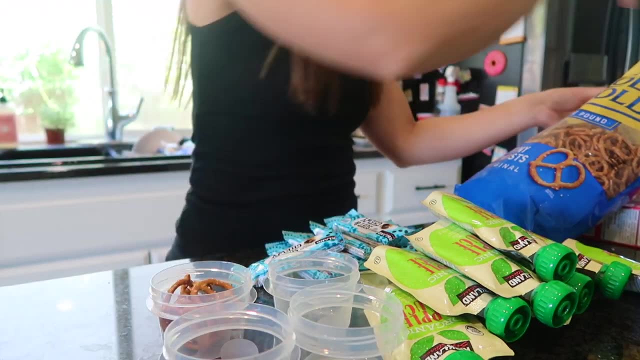 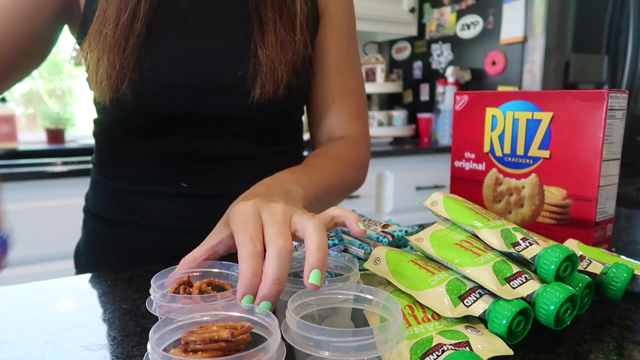 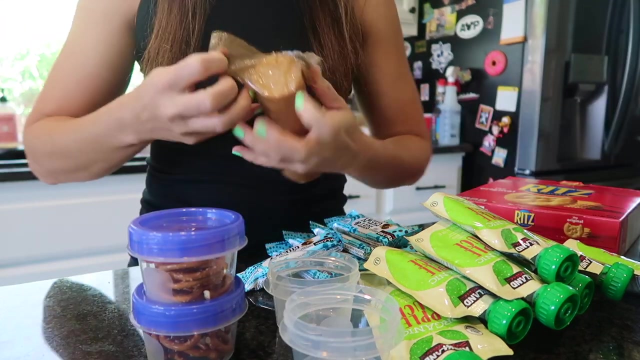 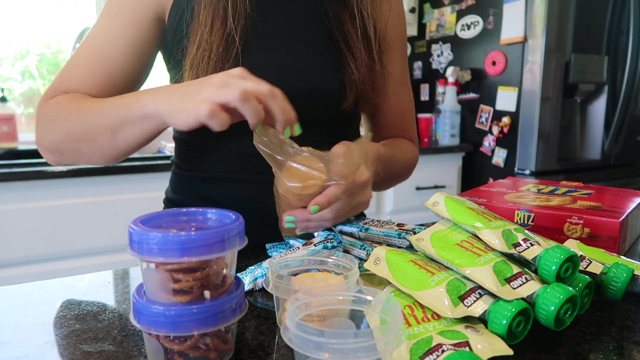 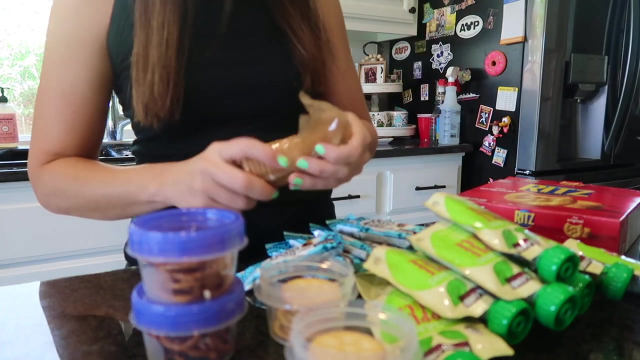 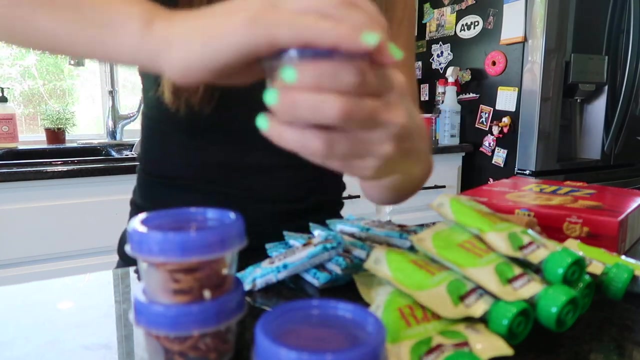 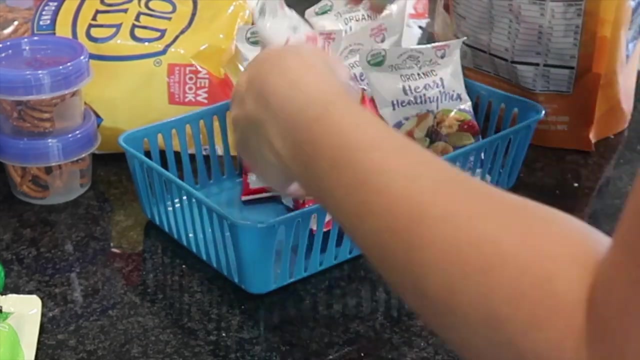 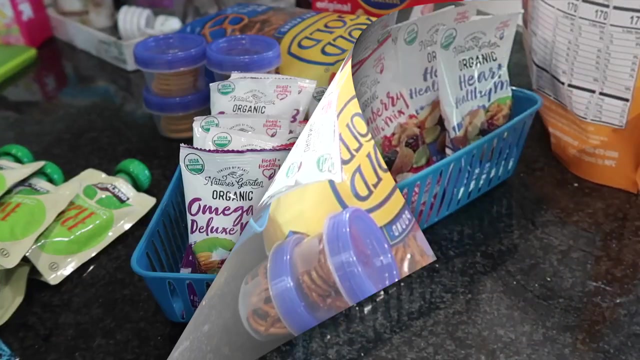 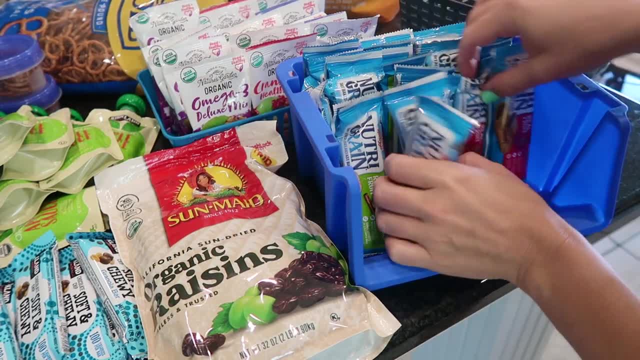 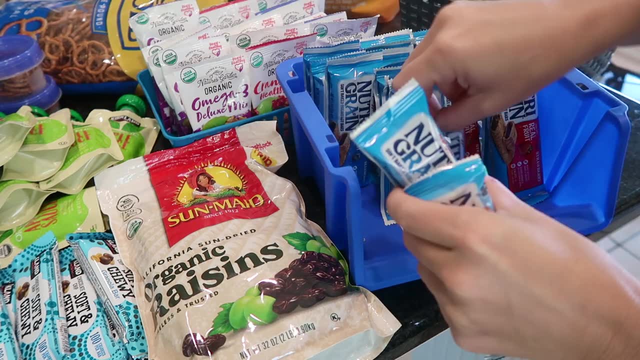 I'm just going to reorganize this a little bit, so it looks a little bit nicer, although they did a pretty good job of keeping it fairly organized. All right, that's better. I'm going to keep these back here. Push these forward. 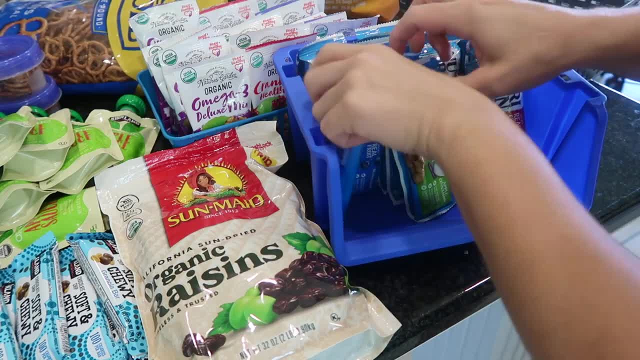 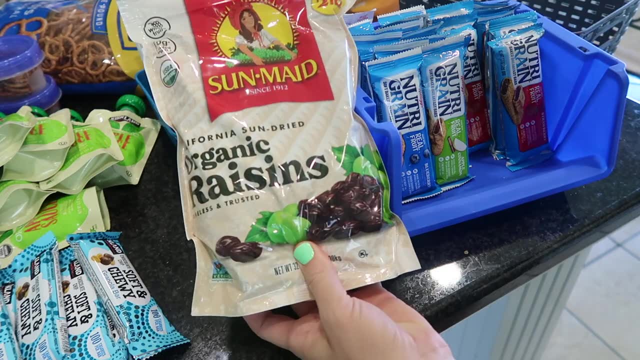 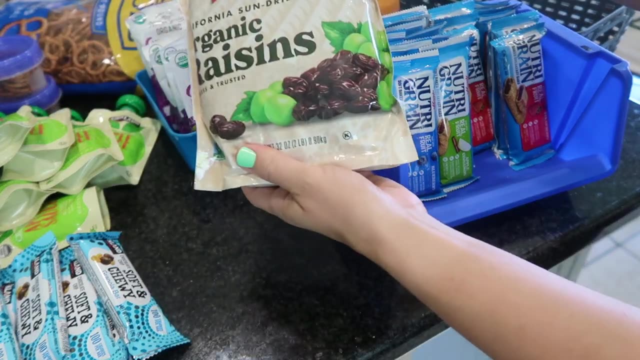 Okay, And I forgot. I had raisins too. So the raisins, I'm going to pre-portion them into little snack baggies and place them next to the crackers and the pretzels. Now, I know that some of these like deluxe mixes have some raisins in it, but I thought that they could also make ants on a log. 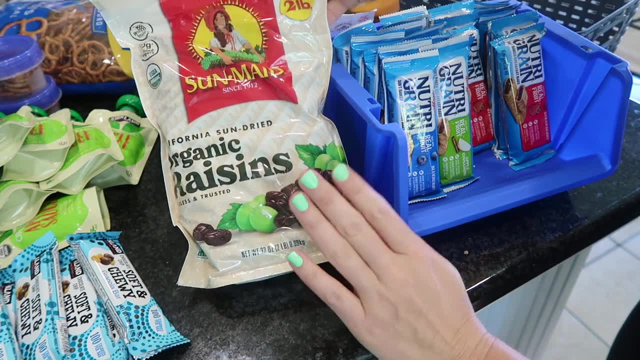 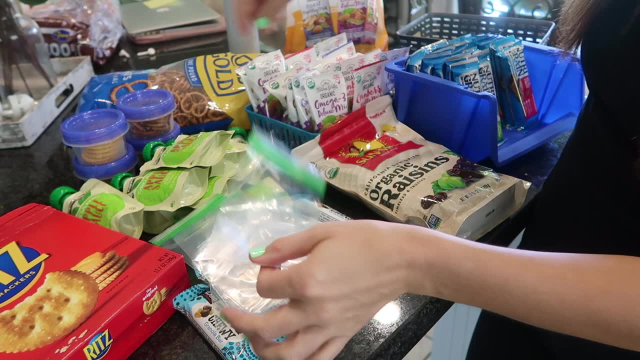 If they decide to get like the celery and peanut butter, they could put some raisins on top. So I want to keep the raisins separate. So, for the raisins, I'm going to use these little snack baggies, And I would be using more of these. 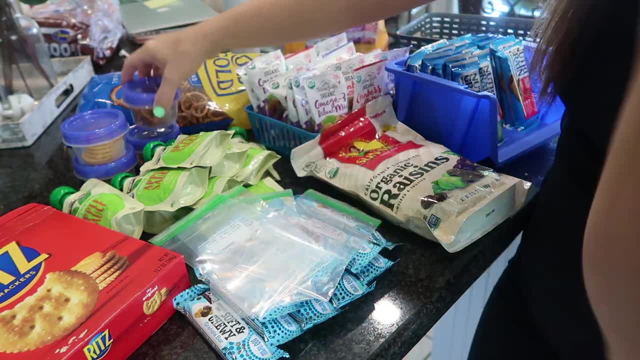 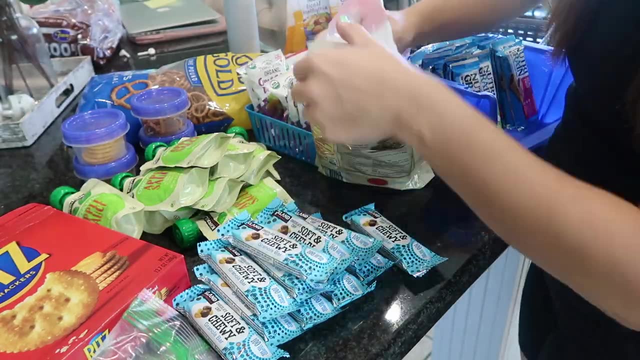 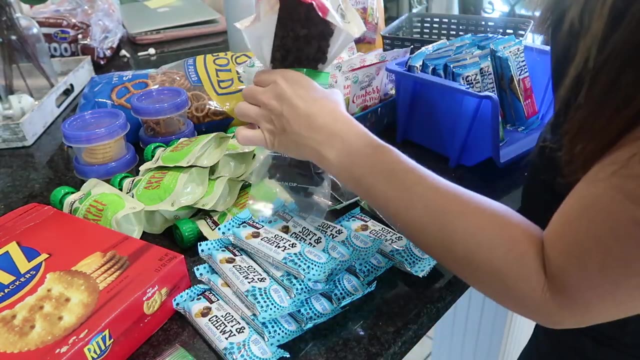 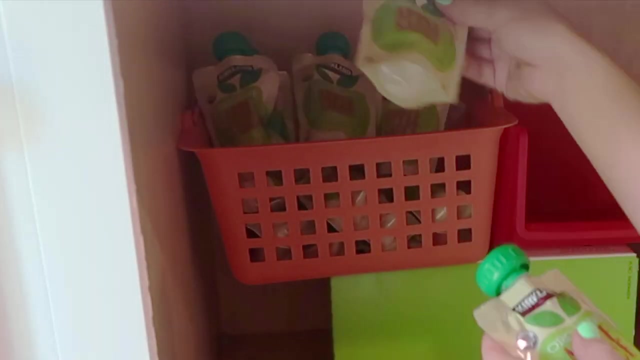 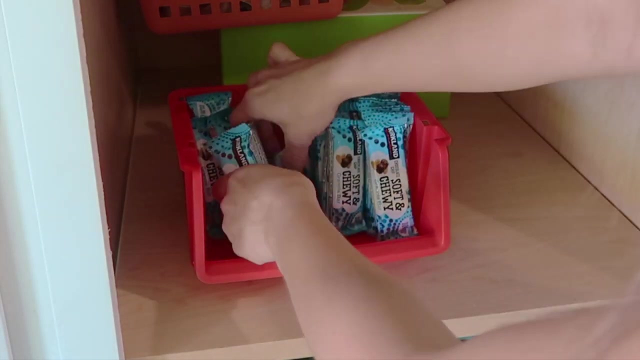 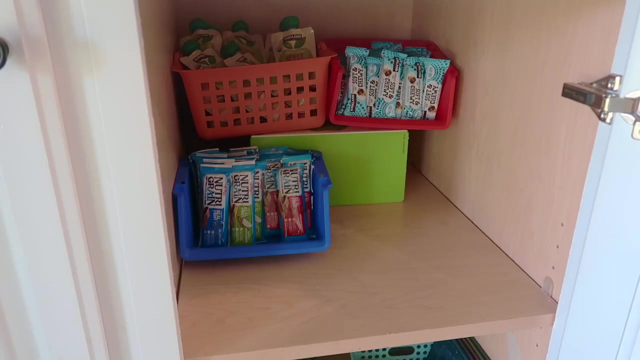 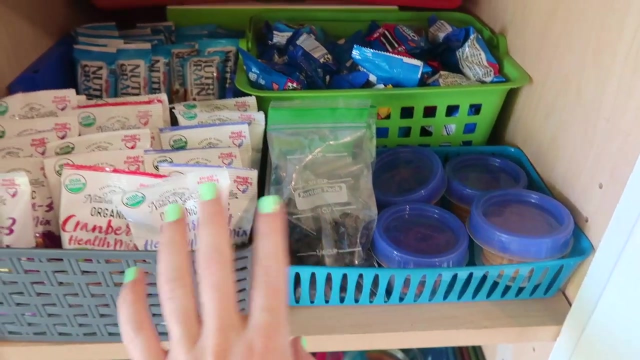 I should get some more of these because I prefer to use, like the reusable stuff, But for now, because that's what I have, I'm going to just put some raisins in here And that's it. I ended up switching the containers around a little bit because these stood. 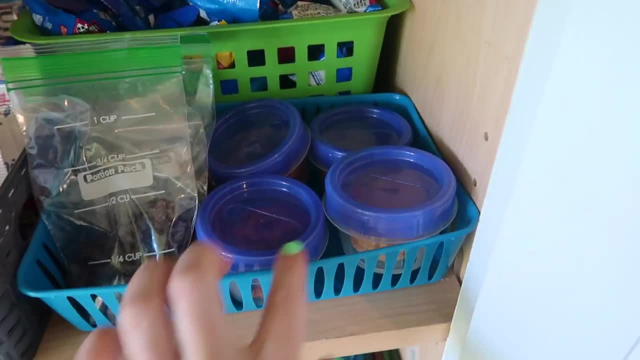 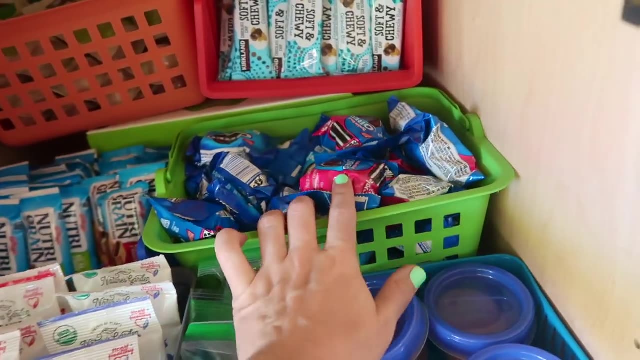 out more and these you could not even see. so I got the pretzels and they have the crackers in here with the raisins, the trail mix, some Nutri-Grain bars, some cookies. they know that you're not supposed to touch unless they ask. 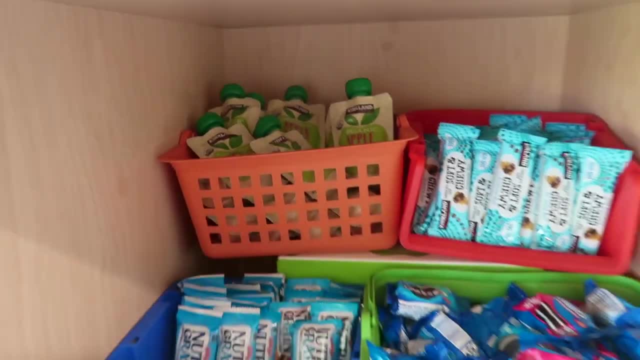 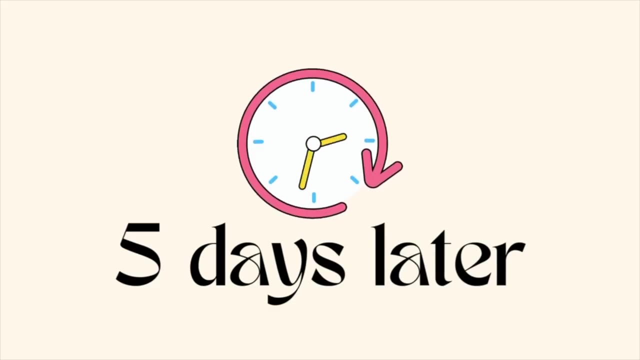 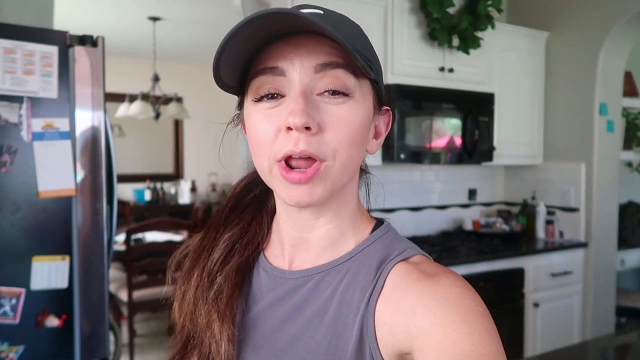 permission for some granola bars and then some applesauce back there. so this is all stocked and ready to go whenever they get home from school. alright, it has been five days since I've done all of the after-school meal prep. I wanted to show you how it turned out, what they loved and what they didn't. 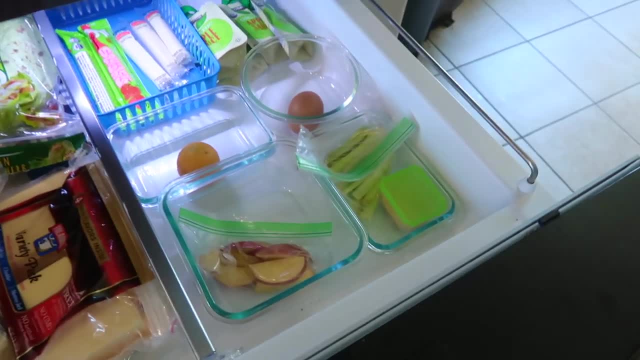 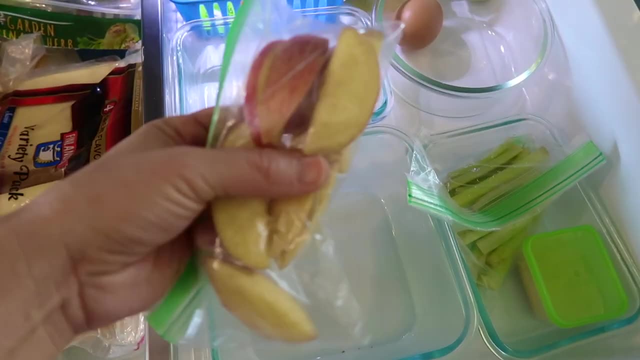 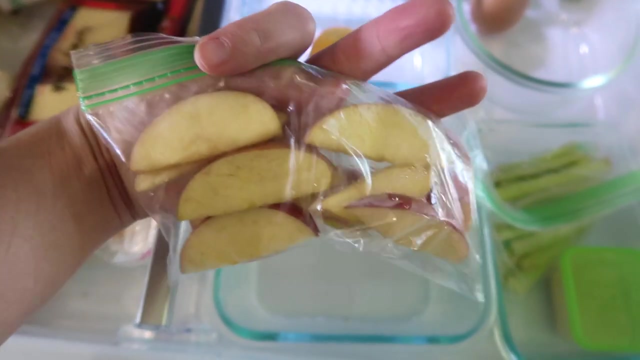 okay, so going right into my fridge first. here is the snack situation in the fridge. apples are pretty much gone. I have one bag left and this is how they look. so is it five days or six days that I'm on? I think it's. I think it's five, but look at how good they don't look that bad. so 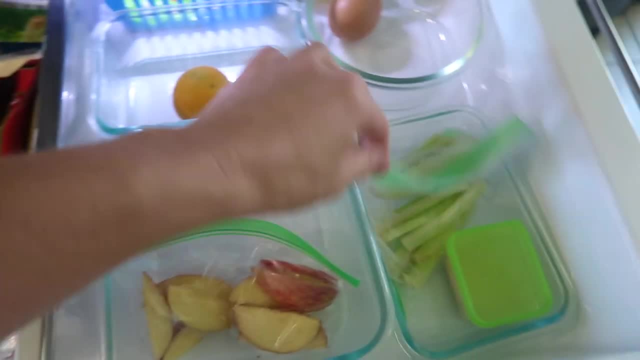 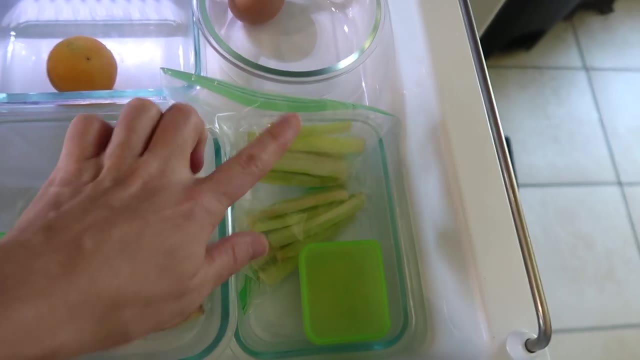 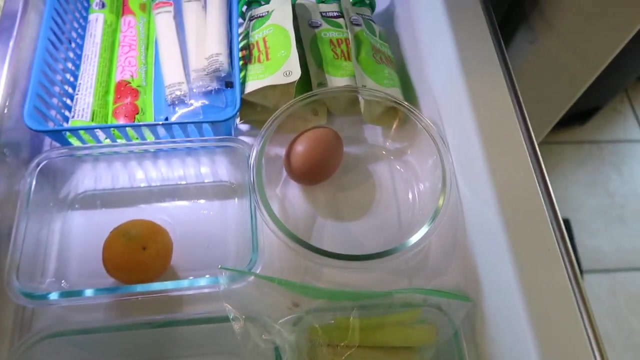 that solution actually really, really worked. so there's that, okay. celery is in. oh, the peanut butter is gone. celery: there's just a little bit of hummus left. I'm probably gonna have celery and hummus for myself. oranges: I had six oranges in here- only one left. I think I had five hard-boiled eggs- only one left. 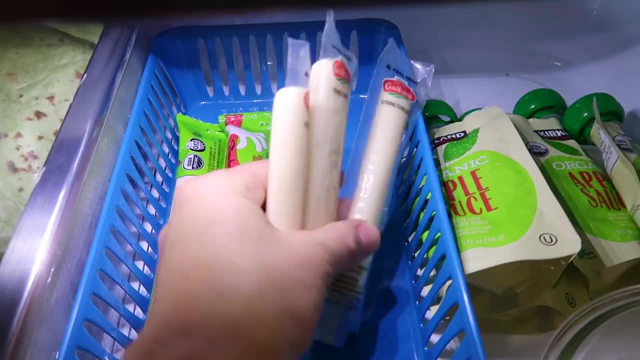 I don't. I don't even remember how many I put in here. I think of the cheese. I just like threw a whole bunch of them in there. I don't even remember how many I put in here- I think of the cheese- I just like threw a whole bunch of them in. 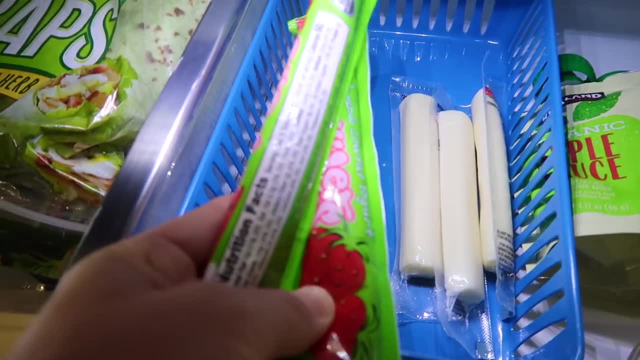 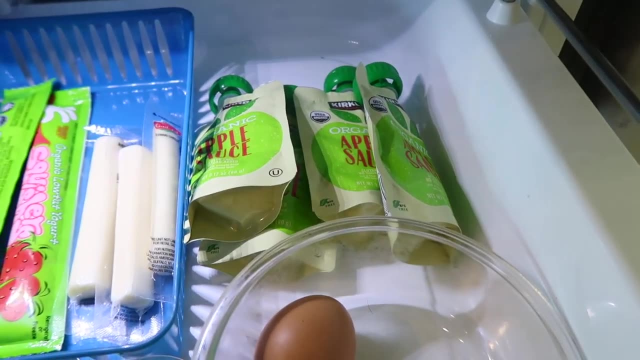 there. I only have three in there. I only have two yogurts left. I threw in a whole bunch in there as well, and then I don't think the yogurt or the applesauce went over as well as it did in the pantry, because I did put some in the pantry too. 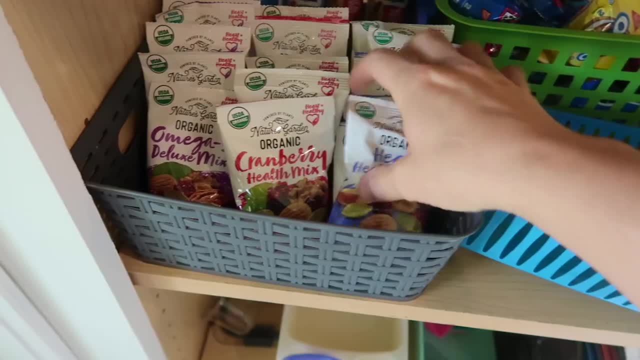 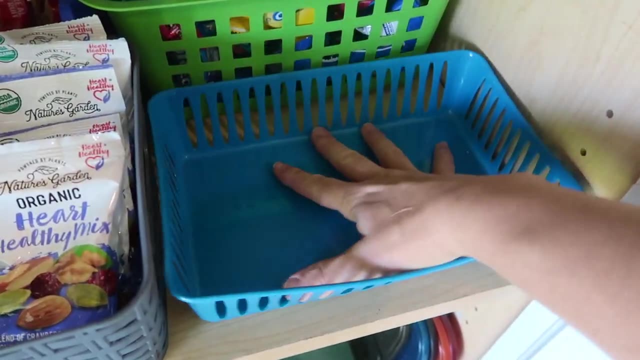 so let's head over there. right now it's yelling at me. some of the nuts are gone because I did reorganize the nuts a little bit more and I did put more in afterwards. so right here I did have like the crackers and the pretzels. here is one. 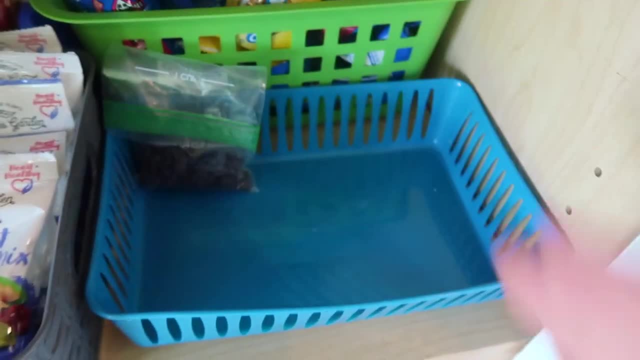 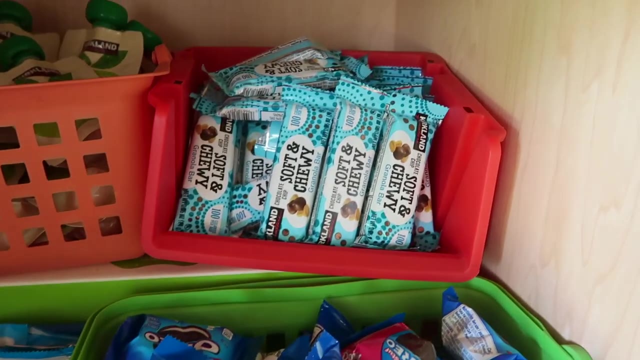 of the raisins. I think I made three bags of raisins, so that's. they did pretty good with this, so they really enjoyed that. there's the Nutri Grains, soft and chewy. I do know some of those are gone, and some of the applesauce back here are gone too, so we're still looking. really 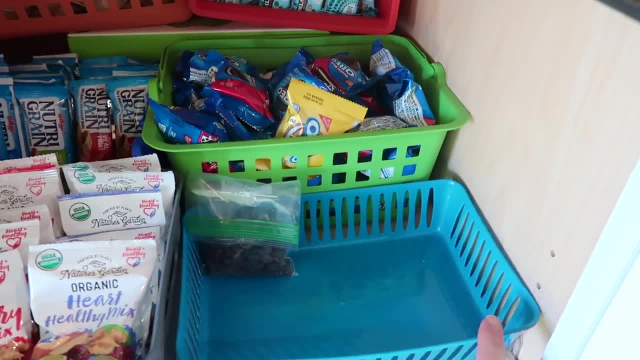 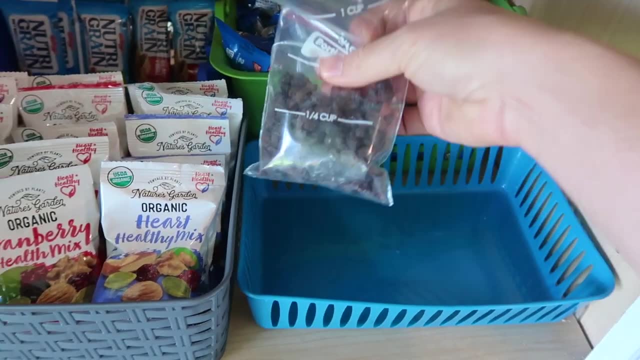 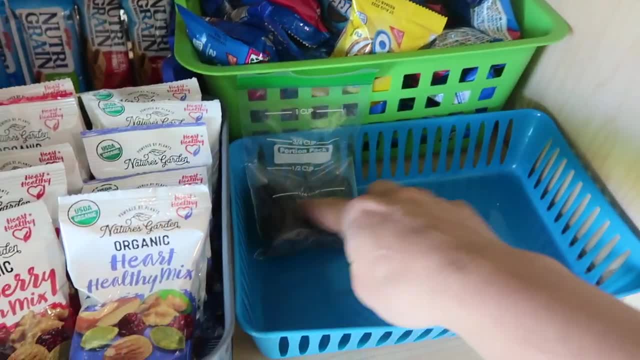 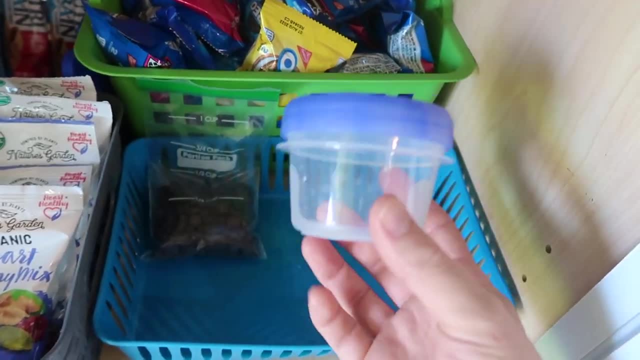 which is probably too many raisins, so I might just get another little baggie and separate them. but what I'm, what I really want to do, is get some more of these little guys or something similar for the raisins, because I don't want to use all. 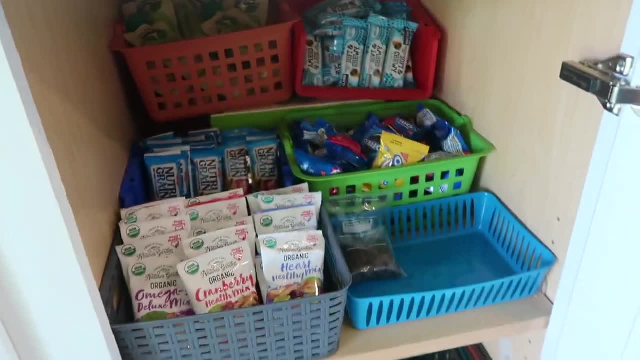 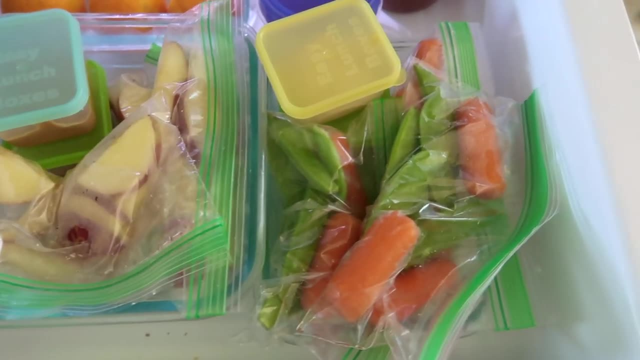 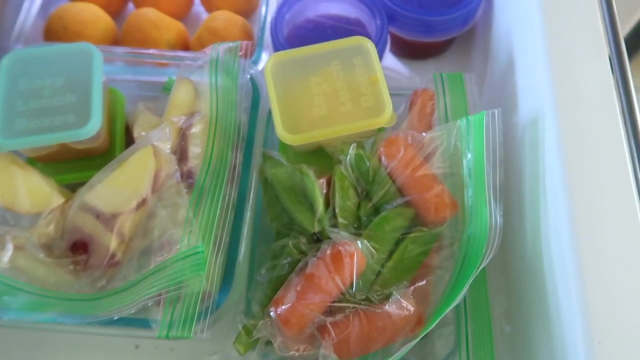 these little baggies, but as far as the snacks go, they really did a good job. I thought I would show you what I restocked the fridge with. so of course I had apples available, so I sliced up some more apples and then for the veggies, I decided to switch it up and do a carrots and the sugar snap peas, and I think they. 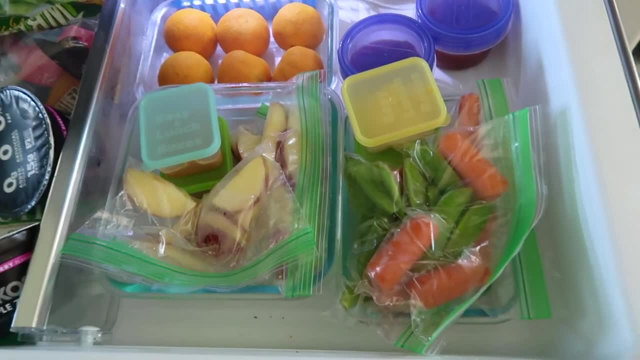 love those more than the pretzels and the pretzels and the pretzels and the more than the celery. so I'm gonna just start doing that until we are all done with the carrots and the sugar snap peas, and then the newest addition I'm doing 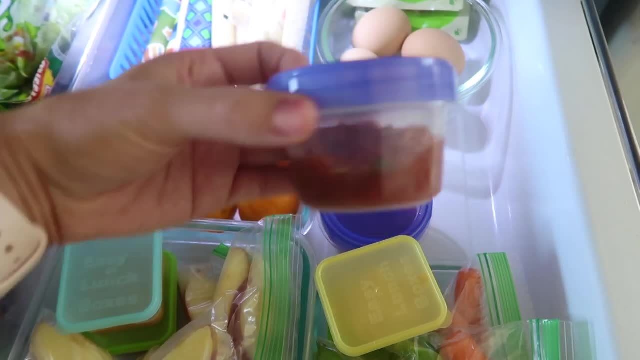 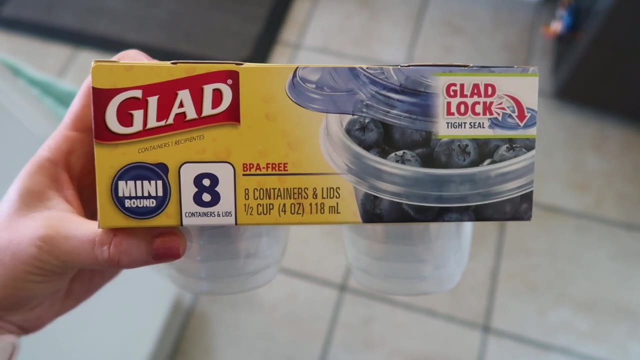 chips and salsa. my kids absolutely love mild salsa, and so I decided to grab some of the containers. now I need to get more, and these are what I picked up. I got them from Amazon. I will link them down below for you, but they're gonna be the. 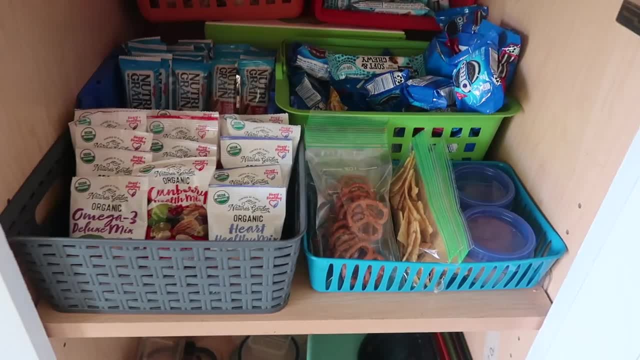 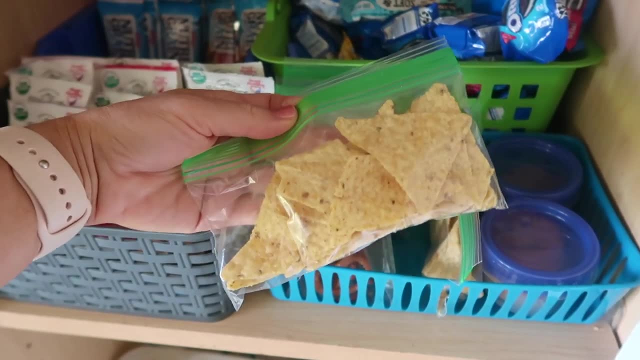 perfect addition. and then for the pantry, of course, I just restocked the crackers and the pretzels and I added some tortilla chips and I added some tortilla chips. and I'm not gonna buy anything new until we were all done with these snacks, because I don't want to waste any food. I don't want anything to. 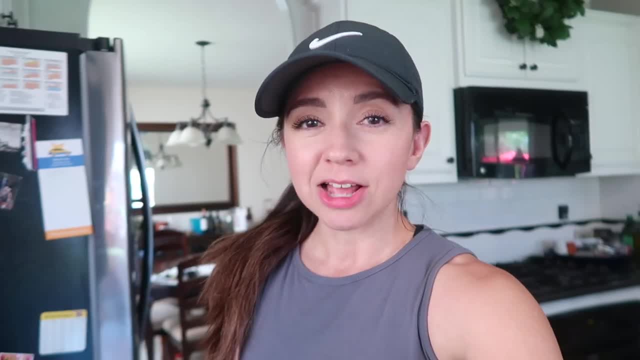 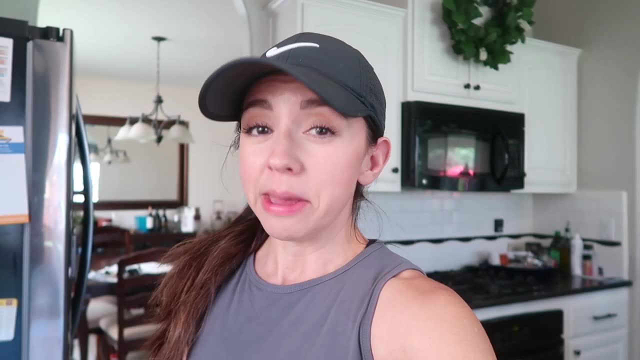 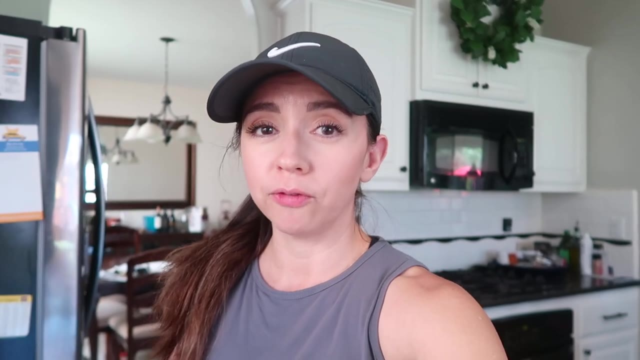 go bad or to go stale. so my thoughts on this after-school prep were phenomenally well. this went really, really good. I loved that. this gave them freedom to choose what they wanted to eat when they came home from school, but also this helped me out as well. I wouldn't have to scramble to figure out. 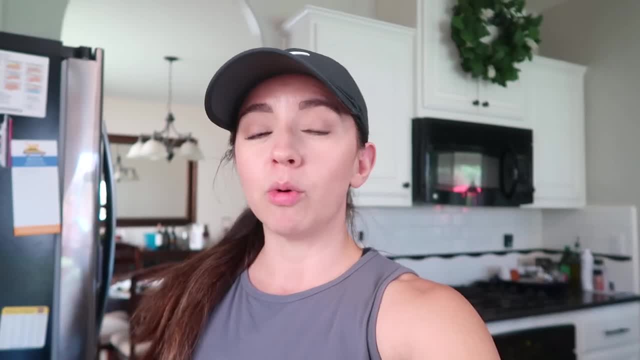 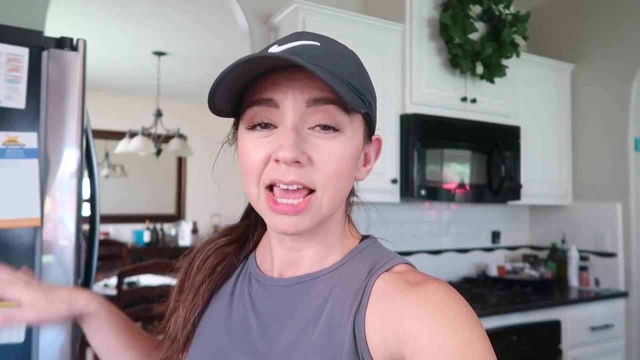 what to give them. so what I'm gonna be doing on Sundays, along with my lunch prep that I usually do, is I'm going to start doing their after school meal prep too. so I'll slice up some carrots, get their little peanut butter cups ready, hummus cups ready, same with the pantry. I'll 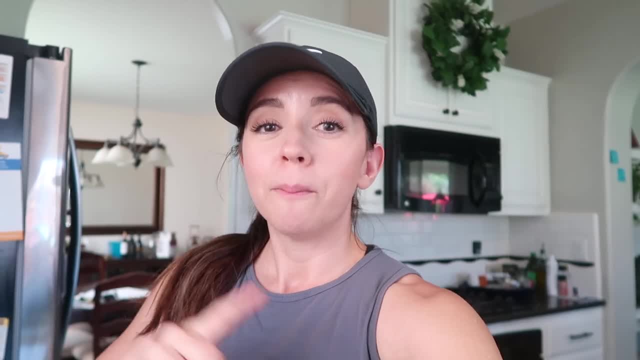 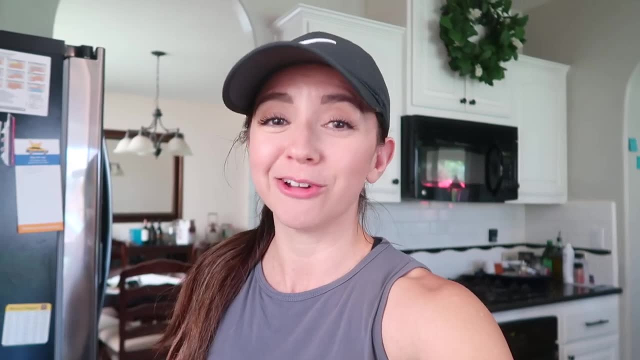 be putting in some pretzels and crackers. so everything is done and good to go. Monday through Friday: everything is set, and I think this is going to help us out in the long run. everybody, everyone's going to be happy, so I really enjoyed this. all right, you guys, and that is it for today's. 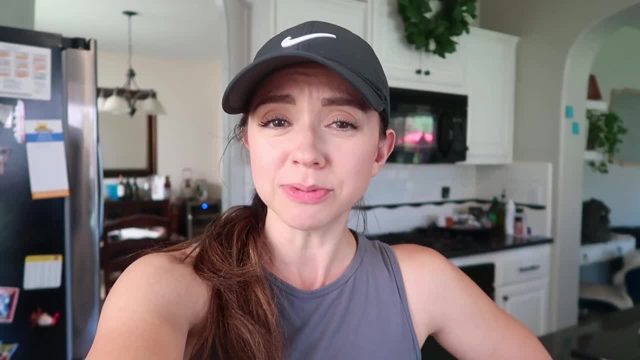 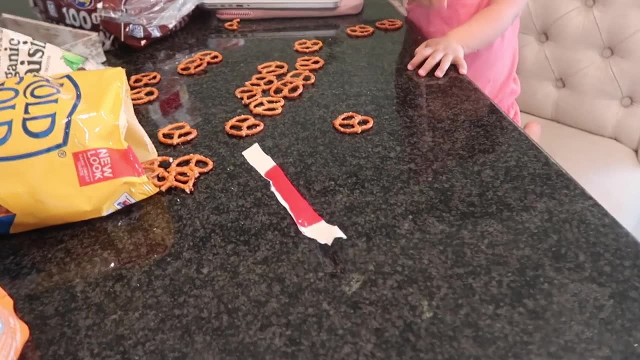 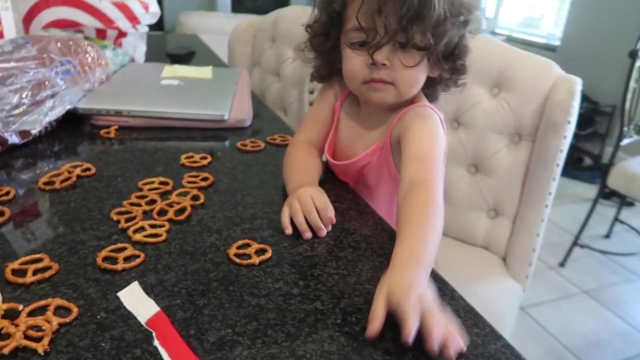 video. if you guys enjoyed it, please give it a thumbs up and subscribe to my channel on your way out. I would really appreciate your support and we will see you in the next video. bye, guys. I turn around for a second and this chick over here- oh, I'm catching the pretzel she's throwing. I'm ready for you to go to school, missus, yay.